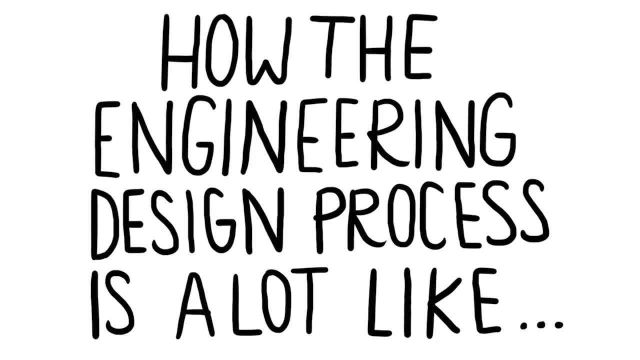 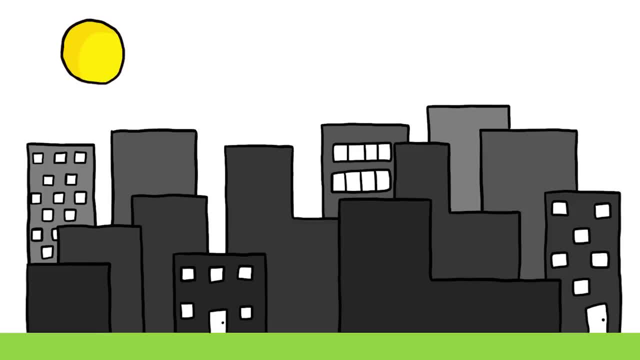 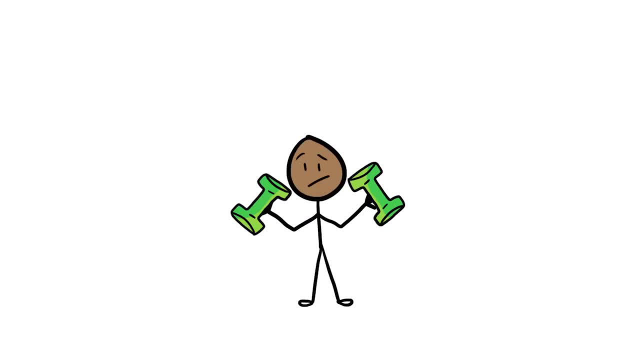 The engineering design process is a lot like making tacos. Here's how Let's say: you've had a long day. Maybe you've gone to class, Maybe you just got off work, Maybe you just finished an intense workout session. It's now 7 o'clock and you're hungry, But you've 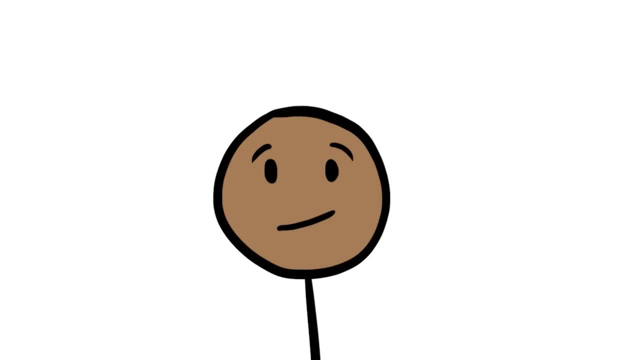 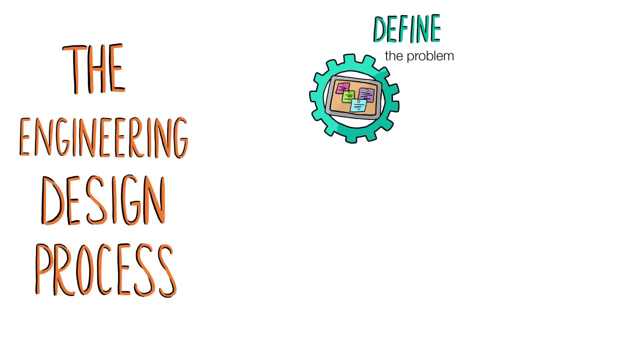 got friends coming over in half an hour. So what do you do? You go through the engineering design process. First, you define a problem or need. In this case, the problem is you're hungry and you've got people coming over in half an hour And they might be hungry too. 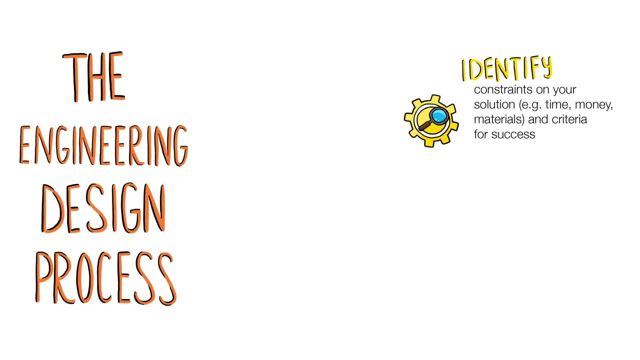 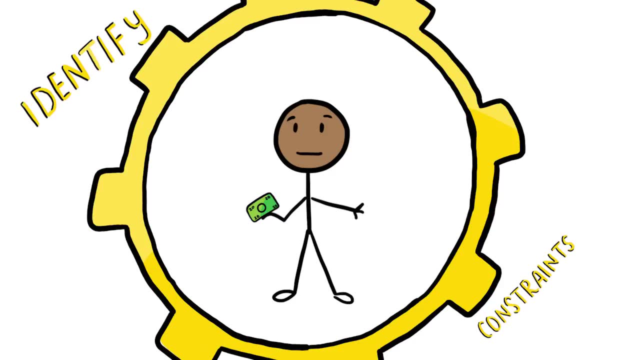 Next, you do some research to figure out the design requirements and your limitations. So in this case, you'd assess things like ingredients. you have at hand, money you've got to spend, how much time you have before people start showing up, how many people you. 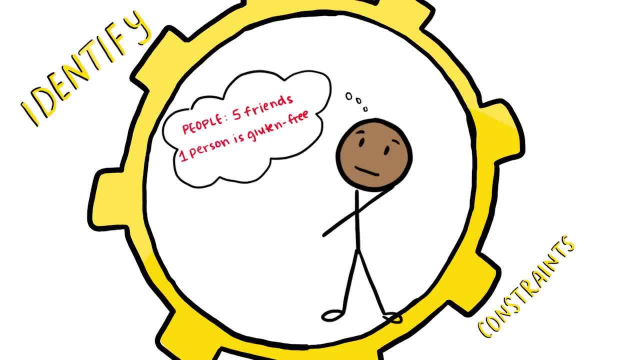 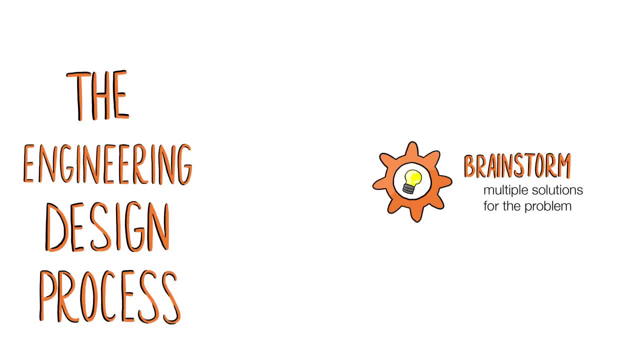 have to feed, and if any of those people have dietary restrictions, Okay, Once you've got a pretty solid list of criteria and constraints, you can start brainstorming ideas for solutions. Maybe you look online at nearby food options. Then maybe you go. 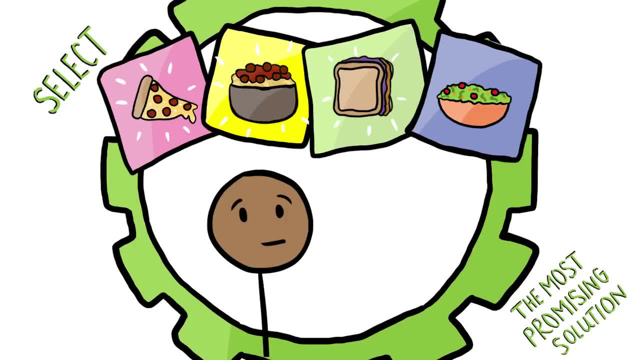 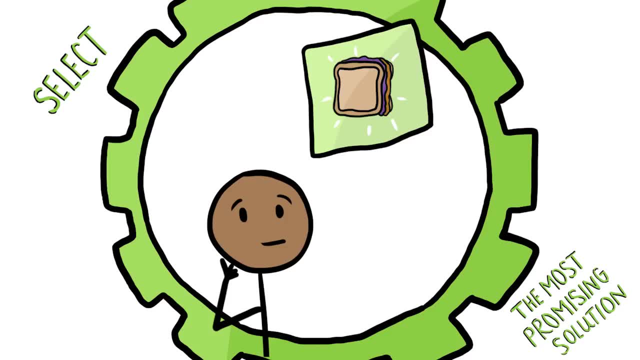 to the fridge and you start figuring out what you can make. You weigh your options and you determine making something at home will be cheaper and faster than ordering something online. And you decide: everyone likes PB&J, but you don't have gluten-free bread. 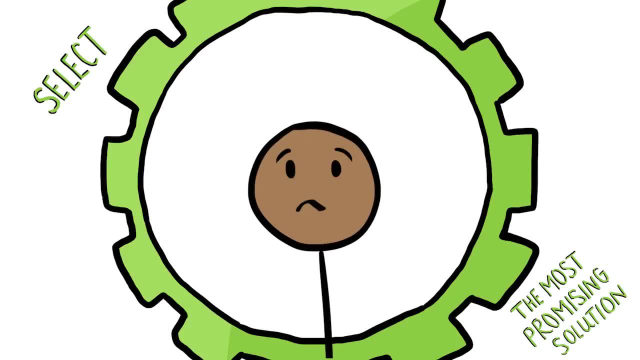 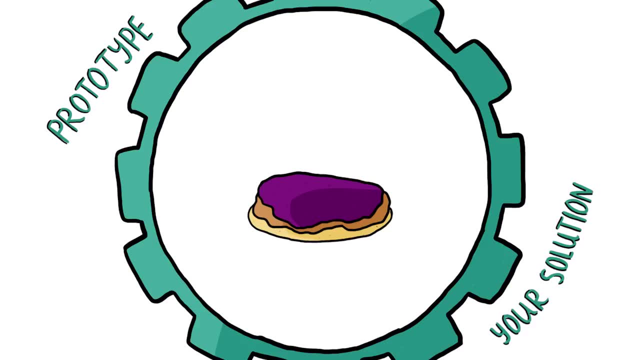 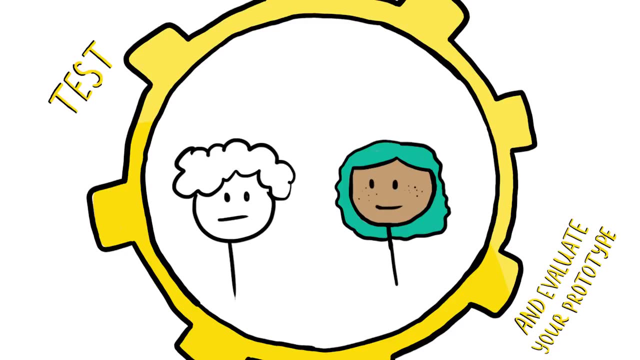 Oh, But you do have corn tortillas. I guess I'll try PB&J on corn tortillas. And you make a prototype, You test out and take a bite. It's gross, But you want to make sure it's not just you, so you get others to test out, like your roommates or family. 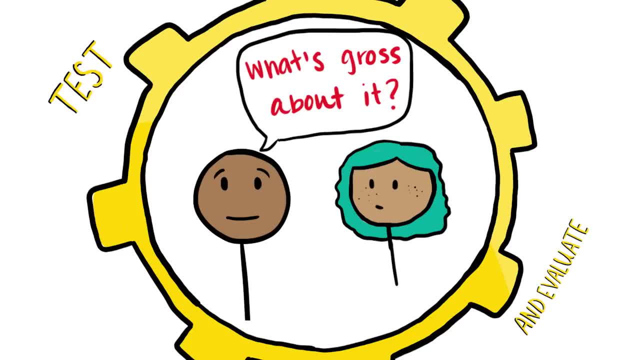 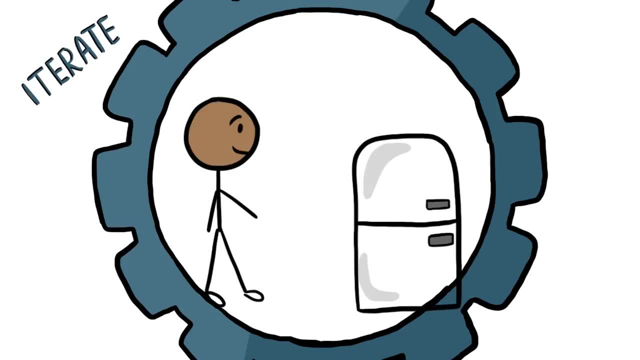 Everyone agrees it's gross. You ask questions and determine what's gross about it. In this case, your testers like the tortillas, but not so much the PB&J. So you go back to the kitchen and reassess. This is what engineers call iterating: making changes based on test and user feedback. You realize.